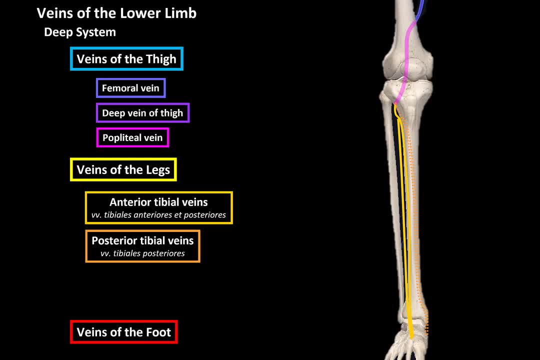 the popliteal vein, The posterior tibial vein splits and becomes these two veins And I tried to be creative here. but keep in mind that the posterior tibial vein lie on the posterior part of the leg and the anterior tibial vein on the anterior side. 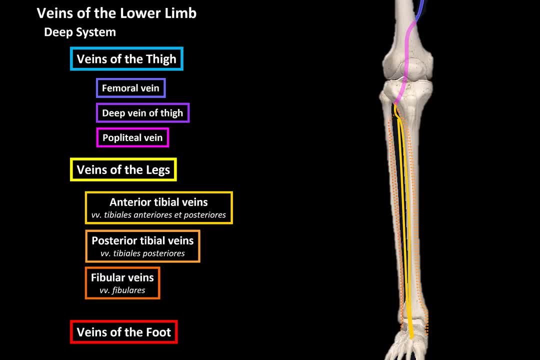 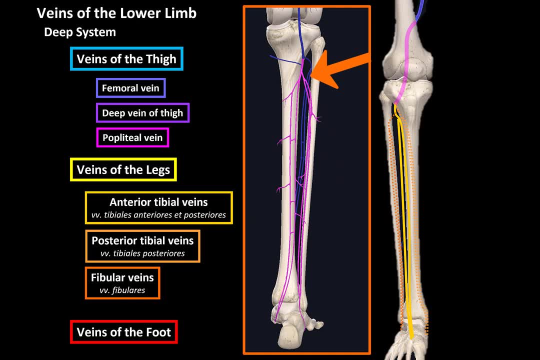 The third deep vein you'll find in this region is the paired fibular vein, which descends behind the fibula, And as you see here, the deep fibular vein is a tributary of the posterior tibial vein, So the posterior tibial veins descend and become the posterior tibial vein. 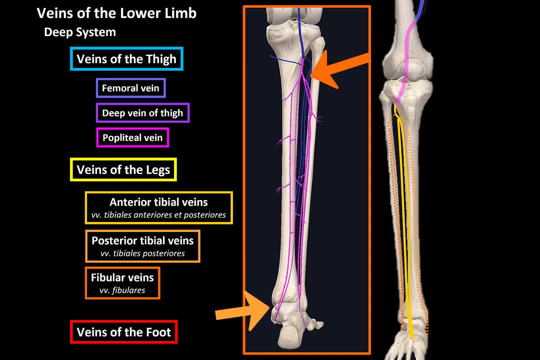 And turn to the sole of the foot behind the medial malleolus. Now, keep in mind that you can always go more detailed than what I'm showing you, but I want you all to gain a general picture of the veins of the lower limb, to ease you all. 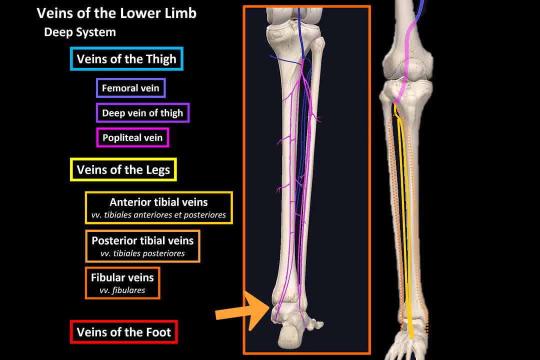 on this topic. So to review, The posterior tibial vein lies posterior to the medial malleolus in the ankle and then it ascends. The fibular vein lies posterior to the lateral malleolus in the ankle and then it ascends. 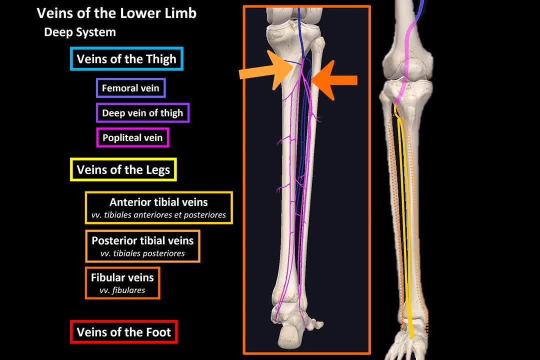 And then it ascends. The posterior tibial vein lies posterior to the posterior malleolus in the ankle and then it ascends, And then it ascends to empty into the posterior tibial vein. So these two are posterior. 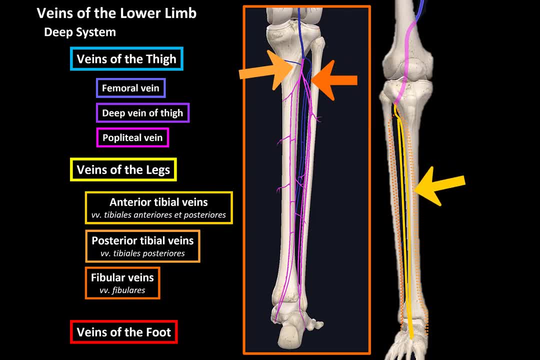 The anterior tibial vein lies on the anterior side. It originates and receives blood from the dorsal venous arch on the back of the foot or the dorsum of the foot, And then it ascends to empty into the popliteal vein. 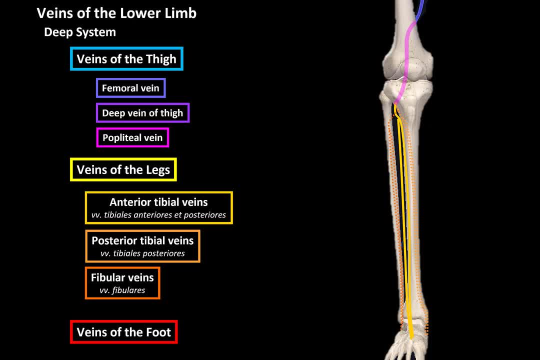 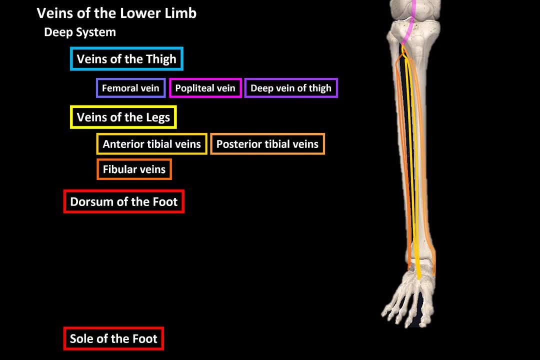 Alright, I hope this made a little sense. Now let's go ahead and do the veins of the foot. These veins are very similar to arteries And we'll divide those into the dorsum of the foot and the sole of the foot. On the dorsum of the foot and now I'm only covering the deep veins, or the most profound. 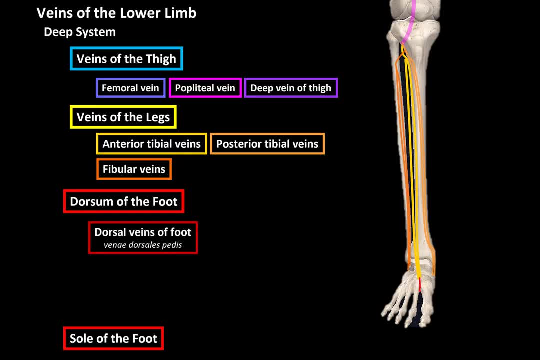 veins you'll find the dorsal veins of the foot. These veins drain a network of superficial veins on the dorsal side of the foot and pump the blood into the anterior tibial vein. And remember, these deep veins always go together with their corresponding arteries. so the dorsal 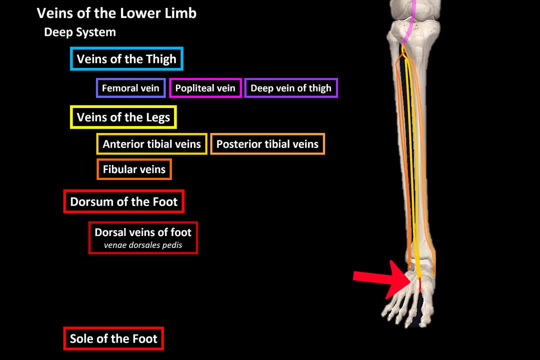 veins of the foot go together with the dorsal artery of the foot. Then, just like the arteries, we got the dorsal digital draining the toes and the dorsal metatarsal veins draining the metatarsals and structures around this region And they pump the blood into the dorsal veins of the foot. 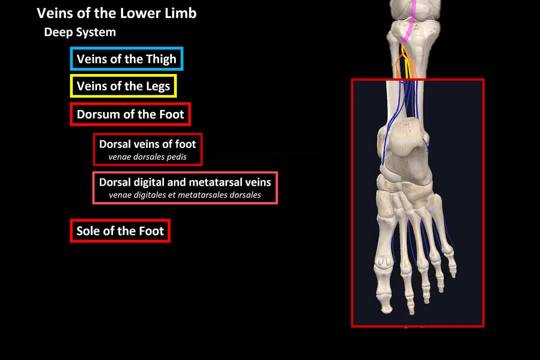 This will make a little more sense in a minute, I promise. On the sole of the foot, the posterior tibial veins will split into the medial and lateral plantar veins, as you see here, And they will form the deep plantar venous arch, as you see here. 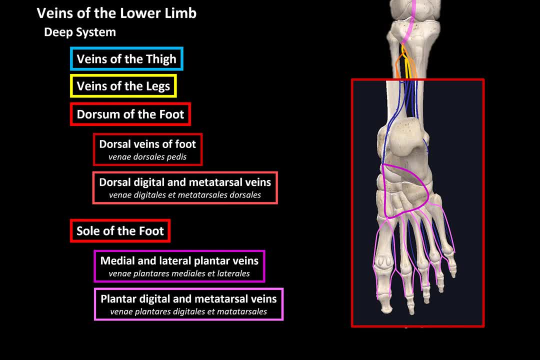 And the deep venous plantar arch will receive blood from the deep plantar metatarsal and the deep plantar digital veins. It's kinda straight forward at this point, isn't it? Let's now go ahead and cover the superficial veins of the lower limb. 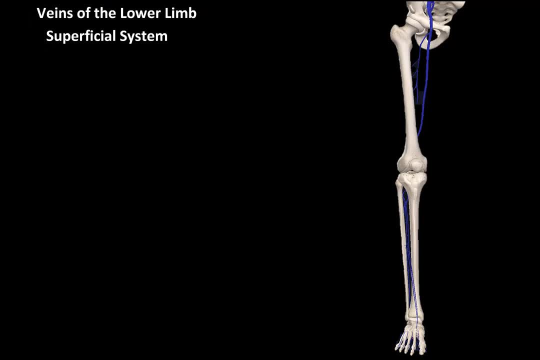 And remember, they lie superficially and they lack corresponding arteries. so they're special for the venous system. And the first one is superficial. It's the great saphenous vein. as you see here, It passes on the medial side of the foot, in front of the medial malleolus and then 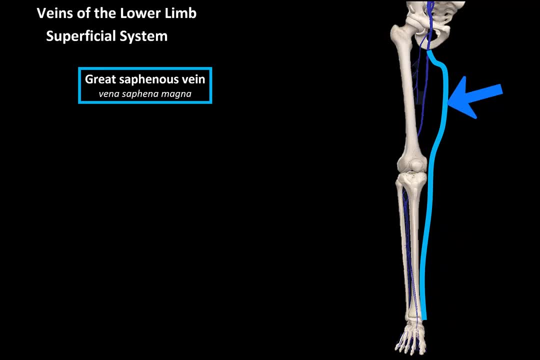 continues on the medial side of the calf On the thigh. it passes through the saphenous hiatus in the fascia lata and then empties into the femoral vein. Now this is a thick vein, so it has tributaries. 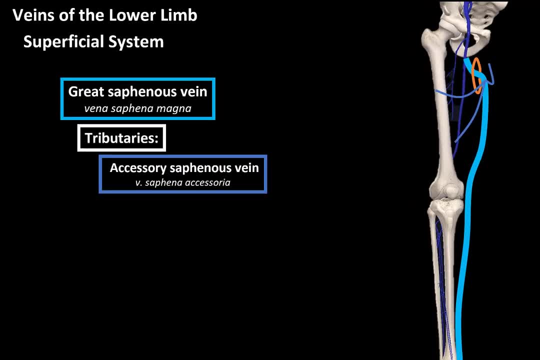 And the first ones are the accessory saphenous veins. as you see here, These veins drain the superficial part of the thigh, It's the great saphenous vein. Then we got a vein that drains the anterior wall of the abdominal cavity, the superficial. 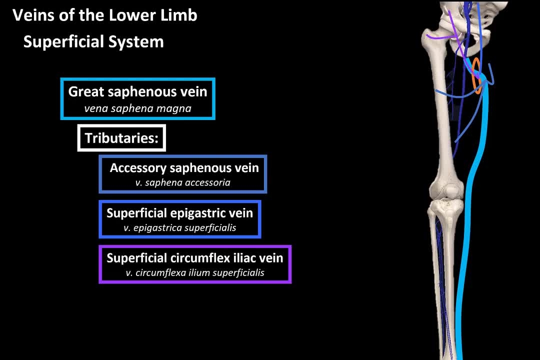 epigastric vein. We got the superficial circumflex iliac vein which passes along the inguinal ligament and drains the regions around the anterior superior iliac spine. And then we got the external pudendal vein. This one is external so it mainly drains the external genitals. so the superficial 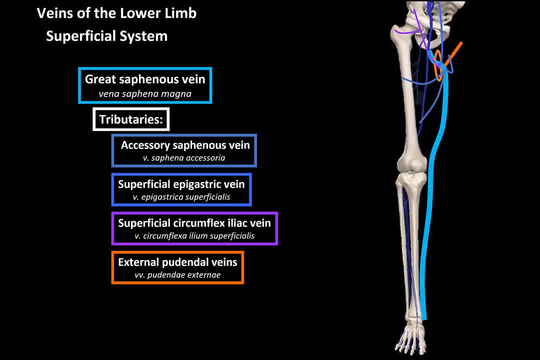 parts of the testis and the penis for men, And then we got the external pudendal vein, which is the external genitals, so the superficial parts of the testes and the penis for men And the superficial parts of the labials and the clitoris for women. 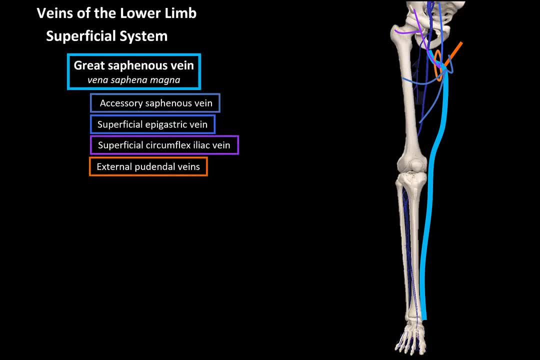 Alright, so that was the great saphenous. Now, since we have a great saphenous, we gotta have a small saphenous vein as well, And this one goes mainly behind the leg, as you see here, Better represented here in purple. 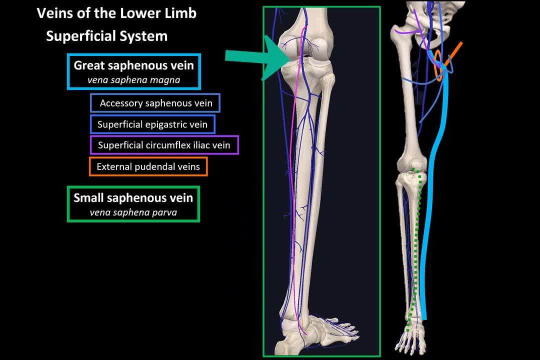 It ascends along the posterior side of the lower leg And then it opens into the popliteal vein, So it mainly drains this area. It also has some accessory branches communicating with the great saphenous vein. It also has some accessory branches communicating with the great saphenous vein. 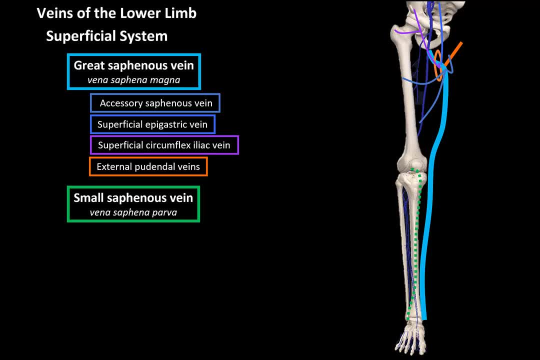 It also has some accessory branches communicating with the great saphenous vein. Awesome. Now next we got the dorsal venous network of the foot. Now, next, we got the dorsal venous network of the foot. This one is relatively straightforward. 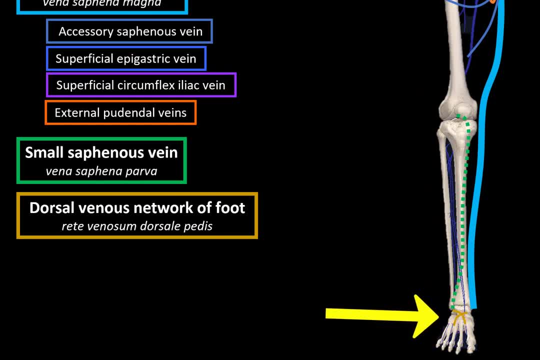 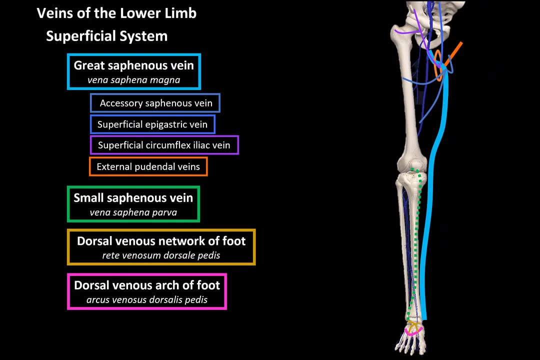 It's just a network of superficial veins on the dorsum of the foot, So it drains the skin and subcutaneous tissue of the dorsal side of the foot And it forms an arch called the dorsal venous arch of the foot. Now, what's unique with this arch is that this arch form the great saphenous vein. 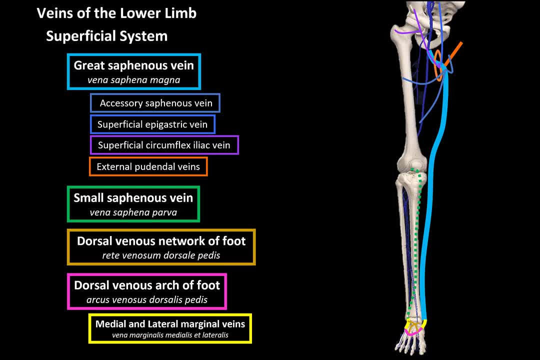 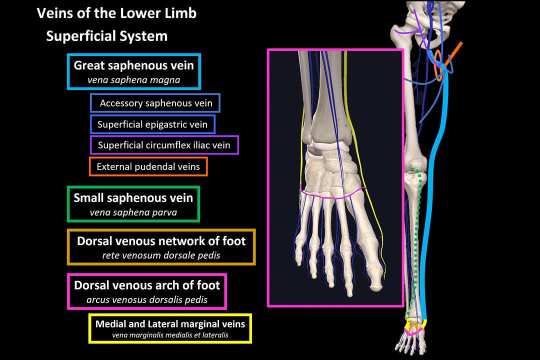 So when you look at your dorsal venous vein, the dorsal venous arch forms the great saphenous vein And then this arch forms the subcutaneous vein saphenous and the small saphenous veins, And it does that through the medial and lateral marginal veins, as you see here. 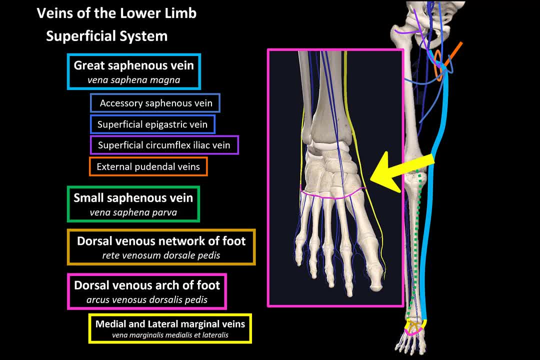 So the medial marginal vein starts off at the dorsal venous arch, then it passes along the medial margin of the foot on the dorsal side and then it continues as the great saphenous vein. The lateral marginal vein also starts off at the dorsal venous arch but then passes. 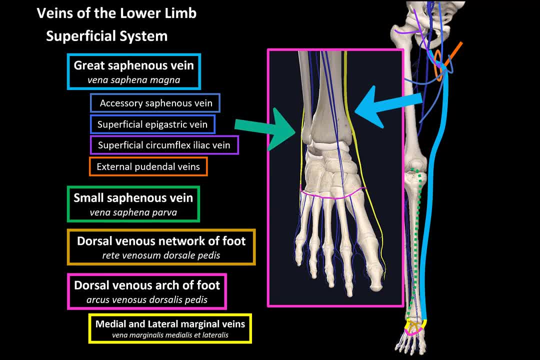 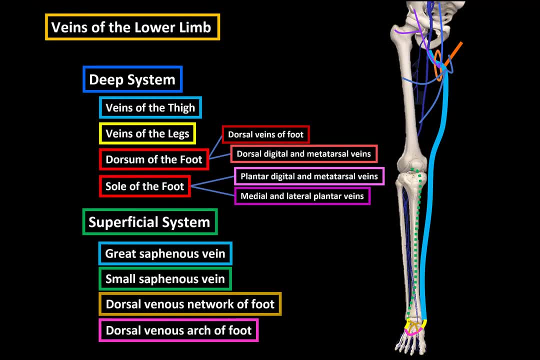 along the lateral margin of the foot and continues as the small saphenous vein. So that was all the essential veins you need to know. regarding the venous drainage of the lower limb, Remember that the deep ones go together with arteries and the superficial ones are special. 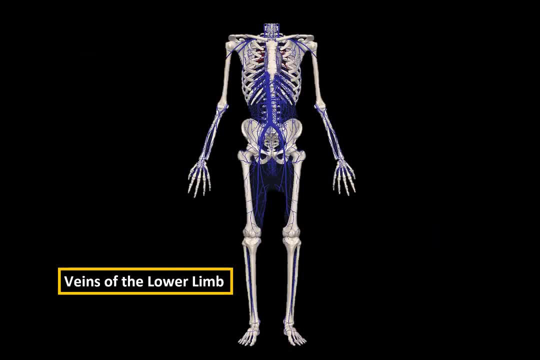 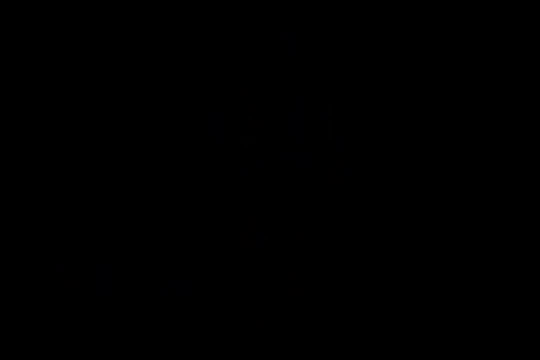 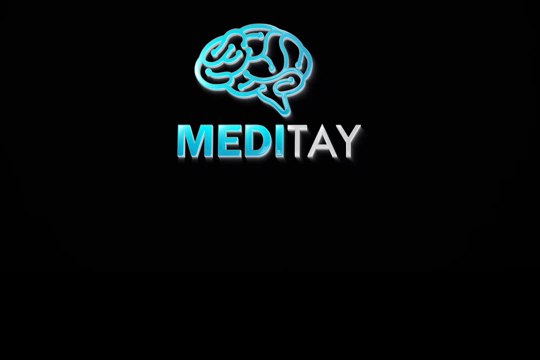 for the venous system. Now the following video will be about the portal venous system. If you found this video helpful, I would really appreciate it if you comment, like and subscribe. See you next time. Bye-bye.